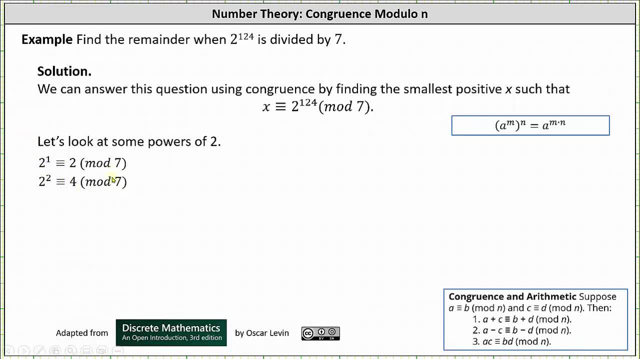 the remainder is two. Two to the second is congruent to four mod seven, since two squared or four has a remainder of four when divided by seven. Next we have two cubed or eight. Two cubed or eight is congruent to one mod seven. 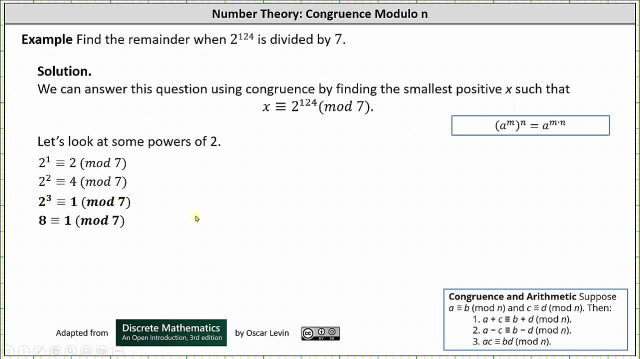 since two cubed or eight has a remainder of one when divided by seven, And this is good news. This indicates every factor of two cubed in two to the power of 124 can be replaced with one, which means for the next step. 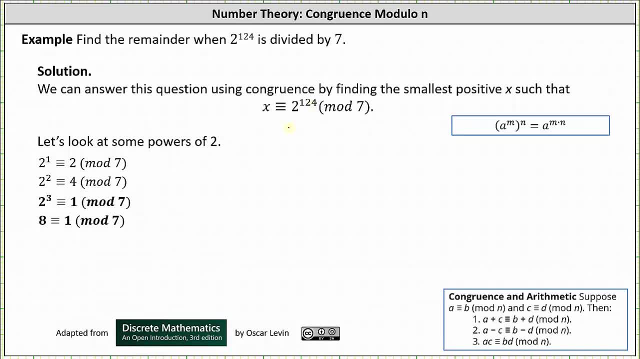 we need to express two to the power of 124 using factors of two cubed. To do this we'll use the exponent property. a to the power of m to the power of n is equal to a to the power of m times n. 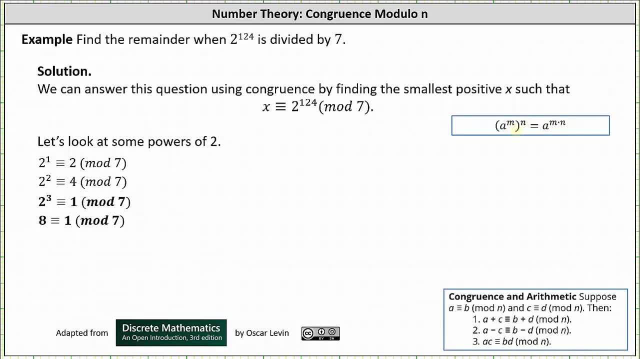 where m is equal to three. To help us do this, we need to determine how many threes are in 124.. To help, let's divide 124 by three. There are four threes in 12.. Four times three is 12.. 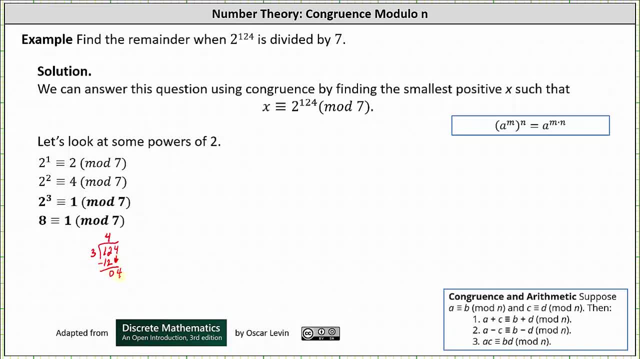 We subtract the difference is zero. We bring down the four: There's one, three and four. One times three is three. We subtract the difference is one. 124 divided by three is equal to 41, with a remainder of one. 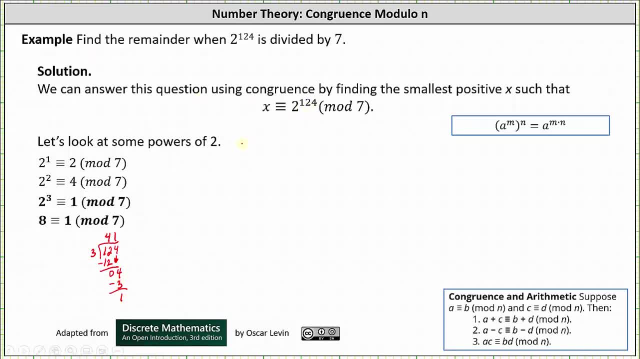 which indicates we can express two to the power of 124, as two cubed raised to the power of 41 times one extra factor of two. Notice, the 41 is the quotient and because we have a remainder of one, we have one extra factor of two. 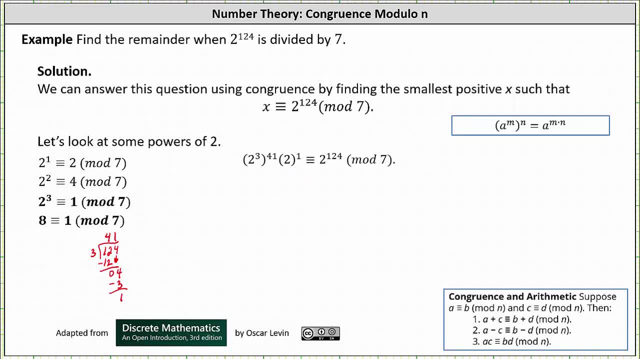 Three times 41, plus one is equal to 124.. And now from here, because we know two cubed is congruent to one mod seven, we can replace two cubed with one. And now, simplifying one to the power of 41 is one. 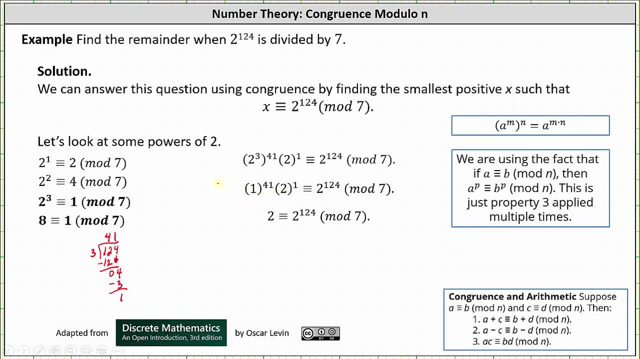 Two to the first is two. One times two is two. We now have two is congruent to two to the power of 124 mod seven, and we're done, because two is greater than or equal to zero and less than seven. We now know when two to the power of 124 is divided by seven.